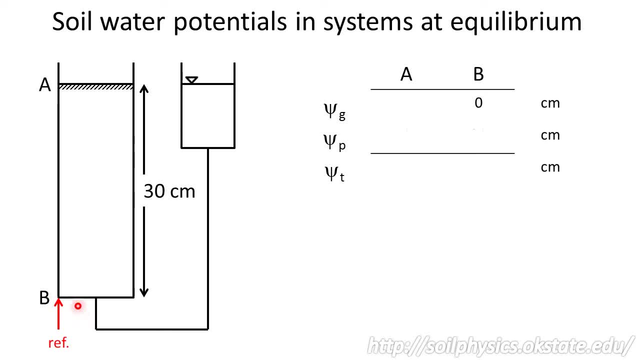 here. here I've chosen but the reference elevation at point B. this choice is arbitrary and it's just made at the bottom here for the sake of convenience. if B is my reference elevation, then by definition the gravitational potential at B is going to be zero. point a is 30 centimeters above my reference. 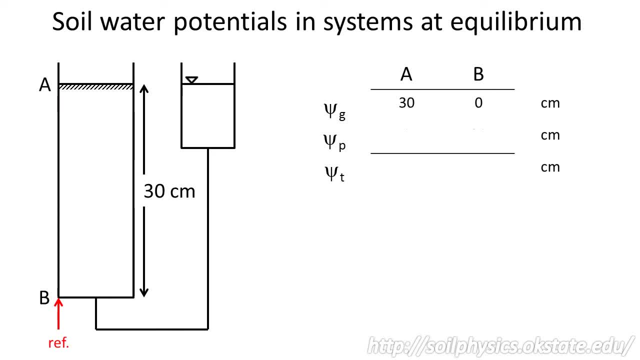 elevation. therefore, the gravitational potential at a will be 30 centimeters, so we can fill that in our table. next we're going to look at the pressure potential at a. notice that a is on the same elevation with and hydraulically connected to the free water. 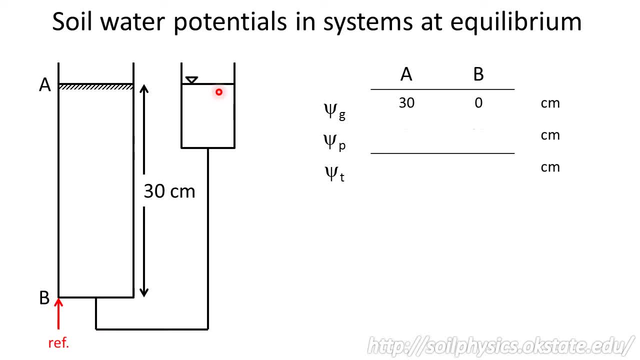 surface. therefore, the pressure potential at a, when this system is at equilibrium, must be equal to atmospheric pressure or zero. the total potential at a, then, is simply the sum of the gravitational and pressure potentials, so that will be 30 centimeters. the total potential at B has to be equal to that. 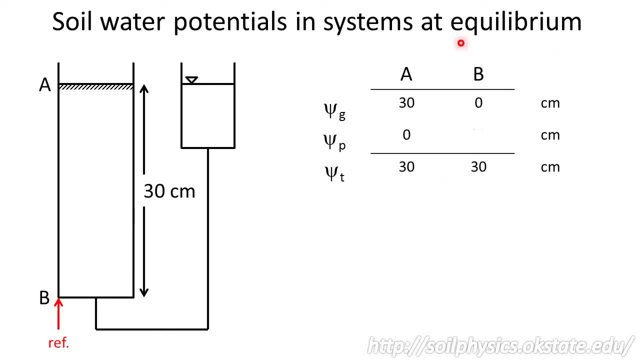 at a when the system is at equilibrium. that's what proof of whatever the equilibrium means, the total potentials are the same throughout the system. so it has to be 30 in both cases. well, now we have only one blank left in our table, and we can see just by quick. 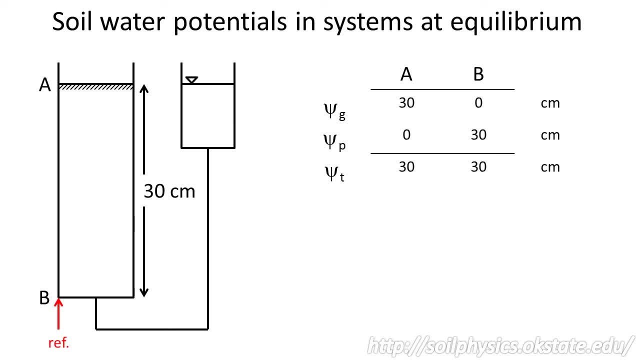 inspection, the pressure potential at point B must be 13 centimeters. that makes sense because it's 30 centimeters below this free water surface and hydraulically connected. so there's our first example. What if we change things up a little bit Now? we've moved the free. 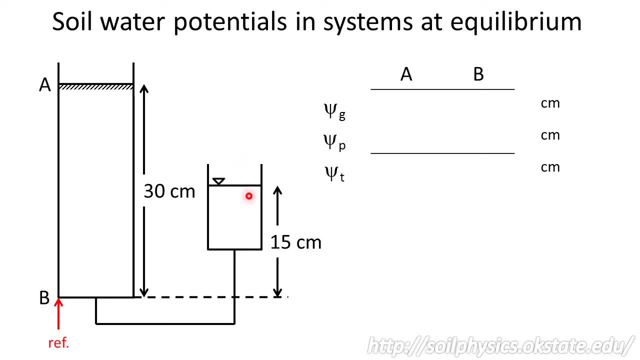 water surface. In this case, the free water surface is only 15 centimeters above the bottom of the soil column. Our reference elevation is still in the same place. Let's see what our table would look like now. Our gravitational potential at B is still zero and our gravitational potential at A is still 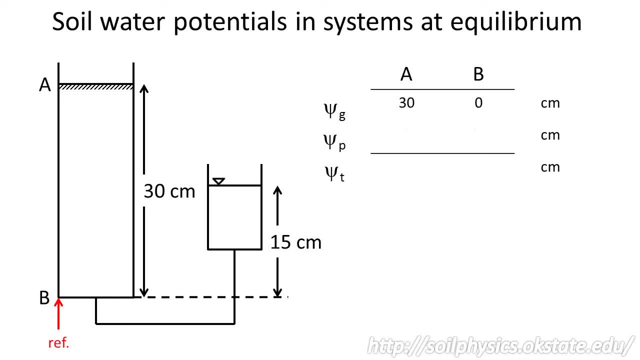 30 centimeters. However, our pressure potential at B is changed. Now the point B is only 15 centimeters below the free water surface, so its pressure potential is positive: 15 centimeters of water. The total potential at B, then, is going to be 15 centimeters of water. 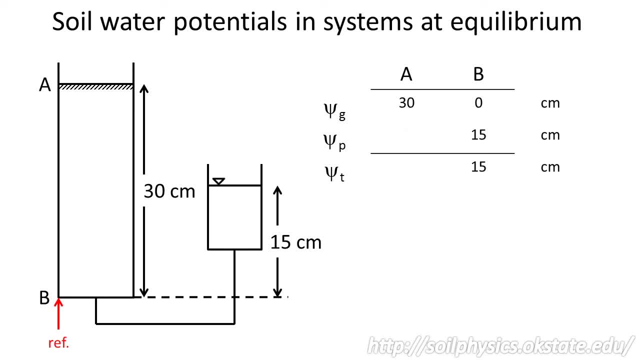 you. And since it's at equilibrium, we know the total potential at A. It is also 15 centimeters of water. Again, by quick inspection we can see what the pressure potential at A must be. It must be 15 centimeters minus 15 centimeters of. 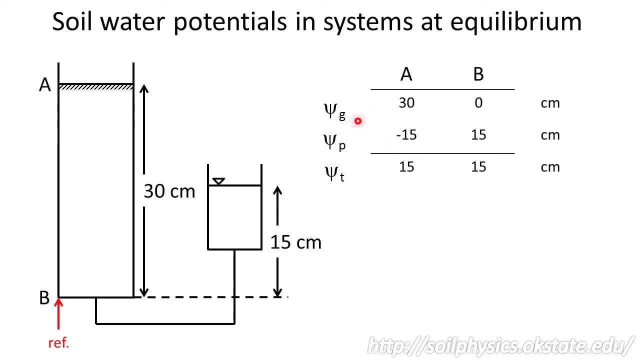 water in this case. So we have 30 centimeters for the gravitational potential, minus 15 centimeters for the pressure potential, giving us a sum of total potential of 15 centimeters. We can continue this and change the example once again by further lowering the water reservoir. Now we have the free water. 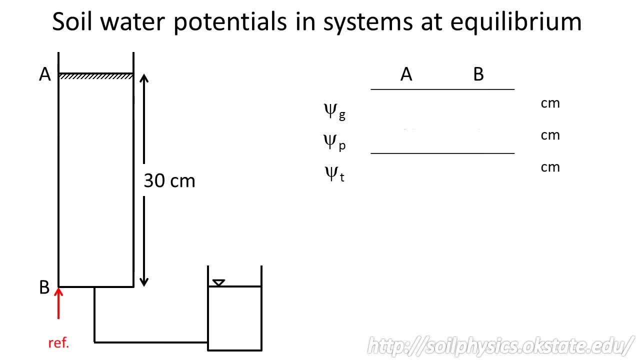 surface equal in elevation with the bottom of the soil column. Gravitational and flight случае. Gravitational potential is always where we start and the gravitational potential at B is zero, at A is 30 centimeters. The pressure potential at B, we know, has to be zero because it's at the same elevation. 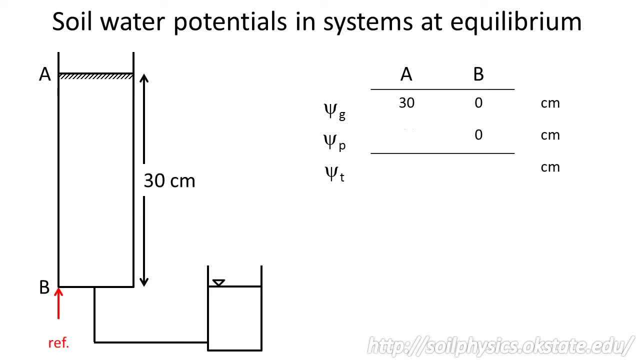 as and hydraulically connected to the free water surface. Therefore, the total potential at B is zero. Since the system's at equilibrium, then the total potential at A is zero. Therefore, the pressure potential at A has to be minus 30 centimeters. 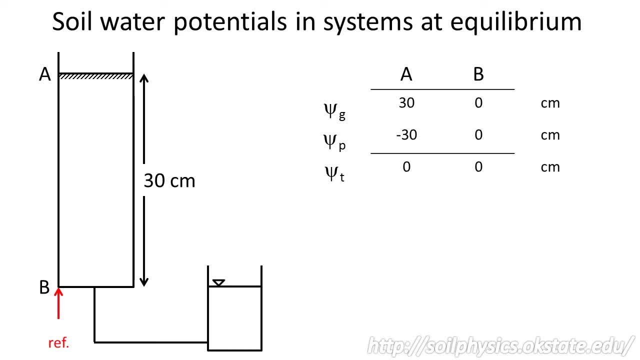 Now I want to make sure you caught one important point regarding the reference elevation. Remember, the choice of the reference elevation is arbitrary. What if we change the reference elevation to be? here? At the end of the video, I'll show you how to do that.